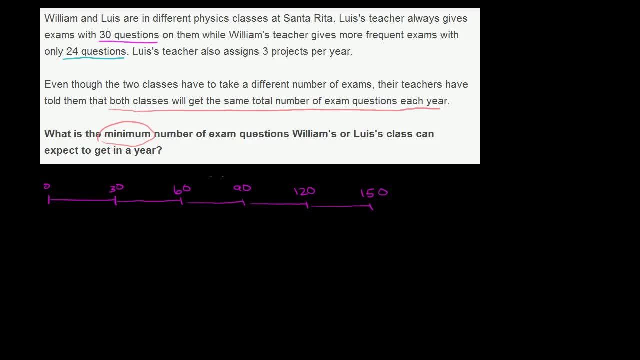 So that's with Luis. Well, what's going on with William Well, William's teacher. after the first test, they're going to get to 24 questions 24.. Then they're going to get to 48 after the second test. 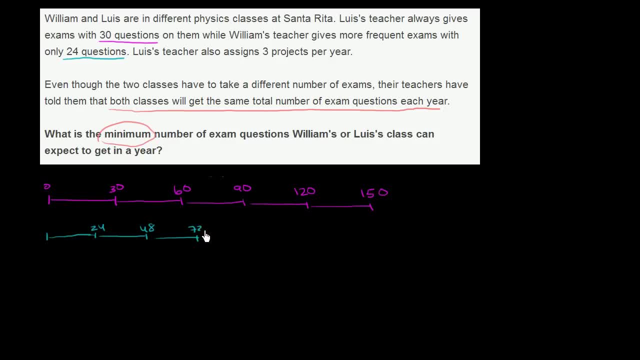 Then they're going to get to 72 after the third test. Then they're going to get to 96.. I'm just taking multiples of 24.. They're going to get to 96 after the fourth test And then after the fifth test they're going to get to 120.. 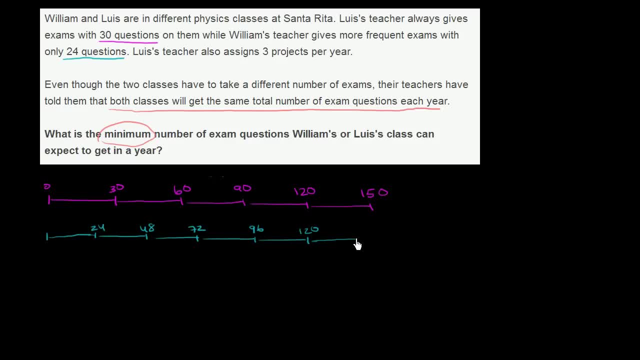 And if there's a sixth test, then they would get to 144.. They would get to 144.. And we could keep going on and on in there. But let's see what they're asking us. What is the minimum number of exam questions? 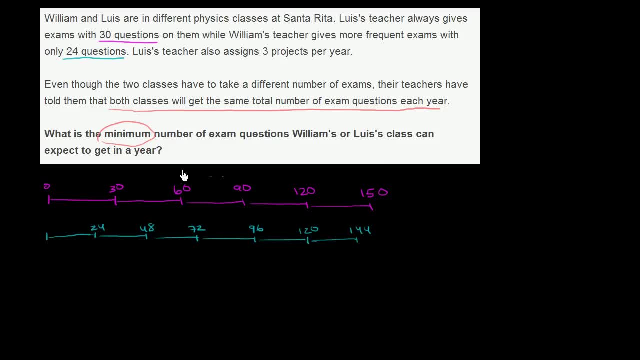 William's or Luis's class can expect to get in a year. Well, the minimum number is the point at which they've gotten the same number of exam questions, despite the fact that the tests had different number of items, And you see the point at which they have the same number. 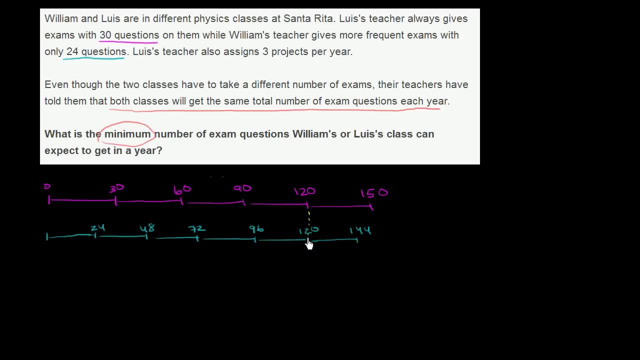 is at 120.. This happens at 120.. They both can have exactly 120 questions, even though Luis's teacher is giving 30 at a time and even though William's teacher is giving 24 at a time, And so the answer is 120. 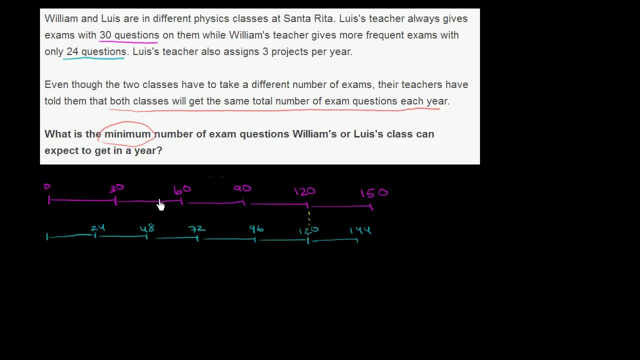 And notice they had a different number of exams. Luis had one, two, three, four exams, while William would have to have one, two, three, four, five exams. But that gets them both to 120 total questions. Now, thinking of it in terms of some of the math notation, 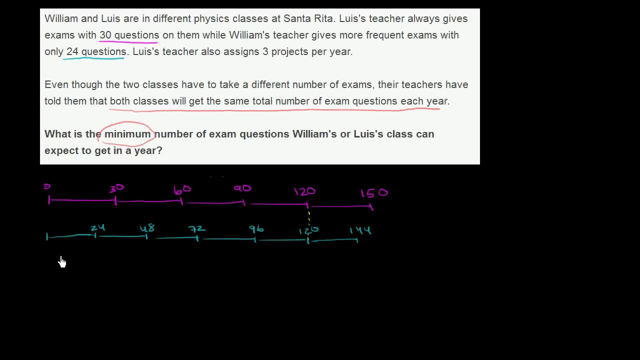 or the least common multiple notation we've seen before. this is really asking us: what is the least common multiple of 30 and 24? And that least common multiple is 120.. So we're going to have to keep going, And we're going to have to keep going. 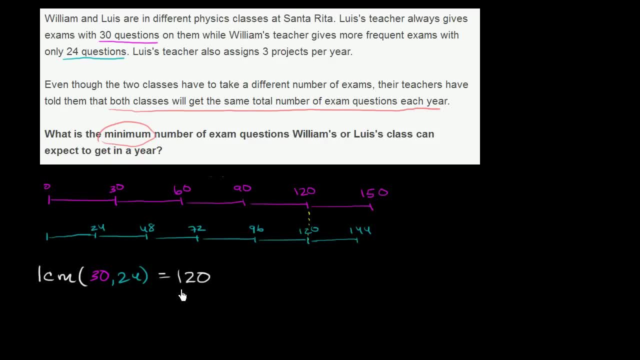 So we're going to have to keep going. So the least common multiple is equal to 120.. Now there's other ways that you can find the least common multiple other than just looking at the multiples. like this, You could look at it through prime factorization. 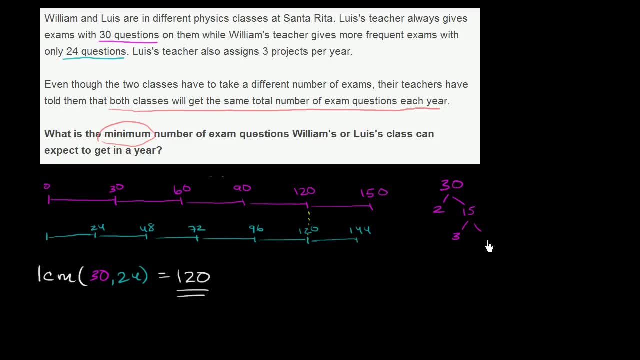 30 is 2 times 15,, which is 3 times 5.. So we could say that 30 is equal to 2 times 3 times 5.. And 24, that's a different color than that blue 24.. 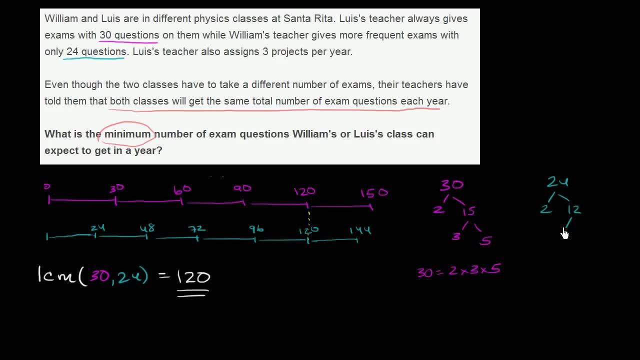 24 is equal to 2 times 12.. 12 is equal to 2 times 6.. 6 is equal to 2 times 3.. So 24 is equal to 2 times 2 times 2 times 3.. 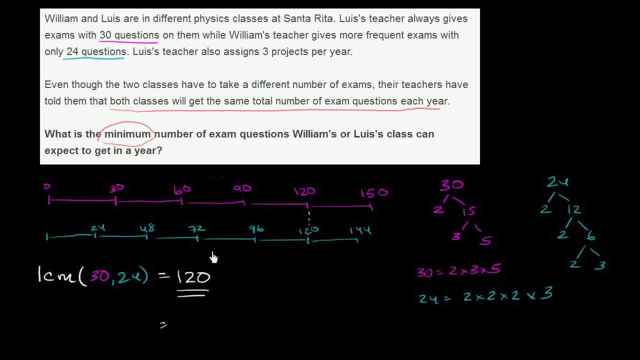 So another way to come up with the least common multiple- if we didn't even do this exercise up here- is: look, the number has to be divisible by both 30 and 24.. If it's going to be divisible by 30,, 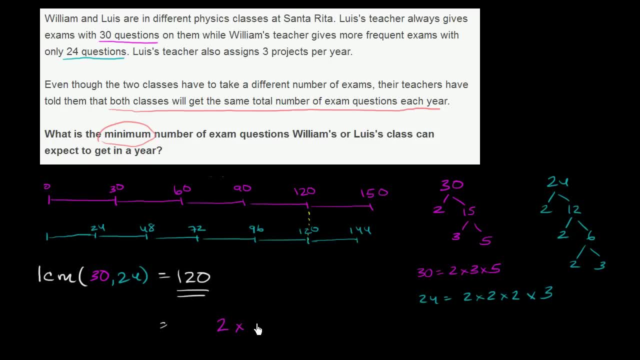 it's going to have to have 2.. It's going to have to have 2 times 3.. It's going to have 2 times 3 times 5 in its prime factorization, That is essentially 30.. So this makes it divisible by 30.. 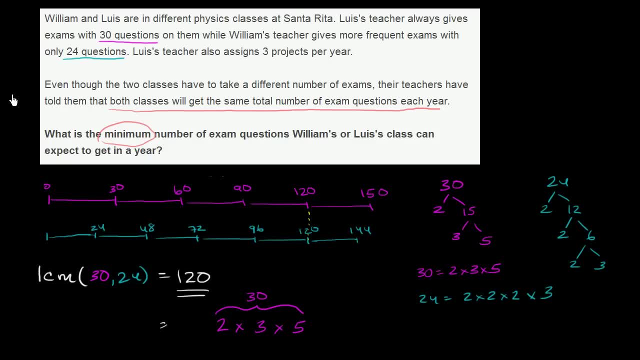 And say: well, in order to be divisible by 24,, its prime factorization is going to need three 2's and a 3.. Well, we already have one 3, and we already have one 2.. So we just need two more 2's. 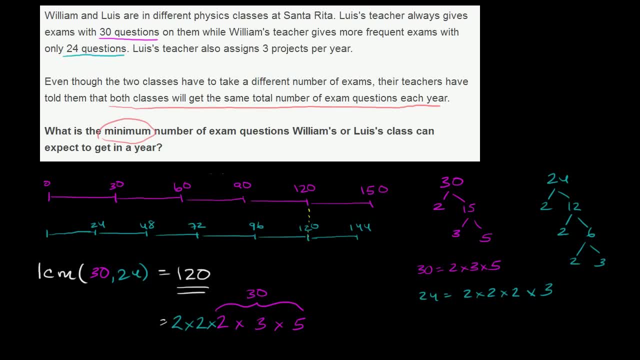 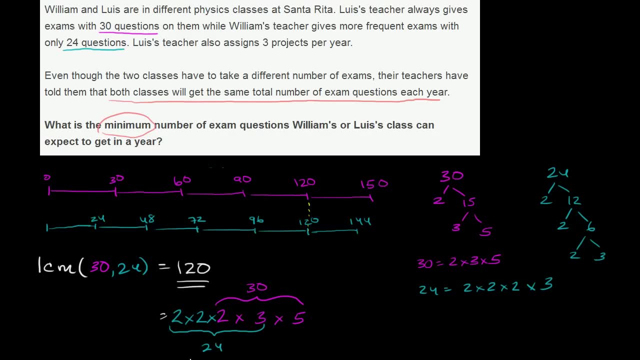 So 2 times 2.. So this makes it- let me scroll up a little bit This right over here- makes it divisible by 24.. And so this is essentially the prime factorization of the least common multiple of 30 and 24.. 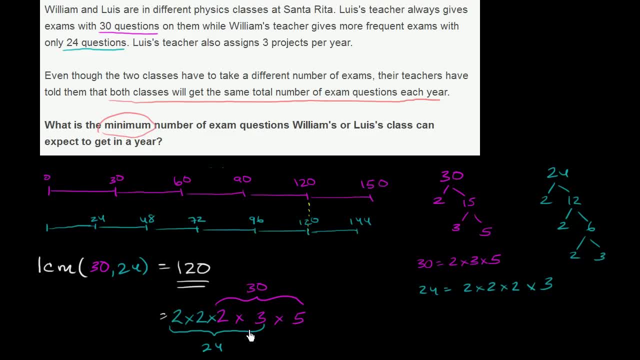 You take any one of these numbers away, you are no longer going to be divisible by one of these two numbers. If you take a 2 away, you're not going to be divisible by 24 anymore. If you take a 2 or a 3 away, if you take a 3 or a 5 away. 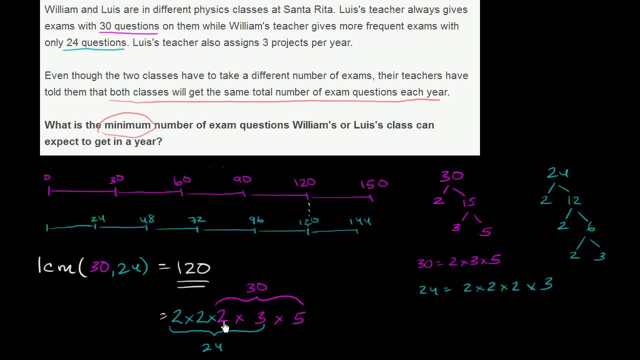 you're not going to be divisible by 30 anymore, And so if you were to multiply all these out, this is 2 times 2. times 2 is 8, times 3 is 24.. Times 5 is 120.. Now let's do one more of these. 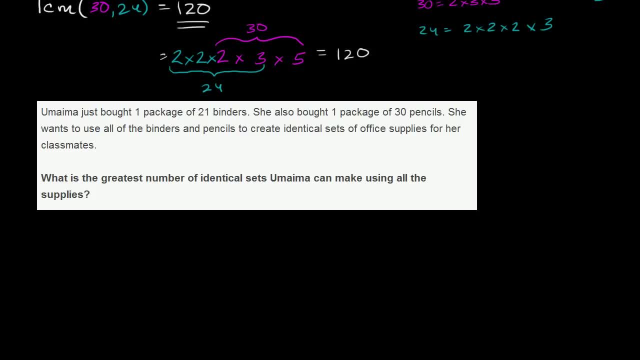 Umama just bought one package of 21 binders. Let me write that number down: 21 binders. She also bought a package of 30 pencils. She wants to use all of the binders and pencils to create identical sets of office supplies. 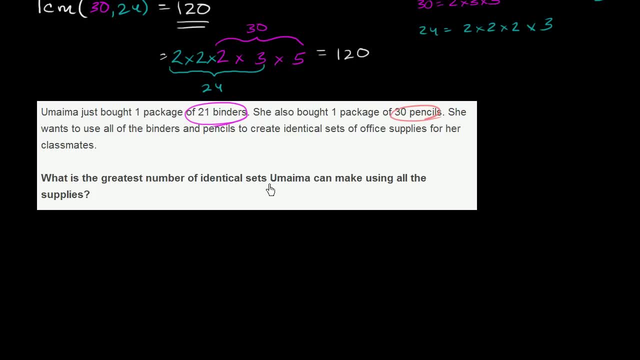 for her classmates? What is the greatest number of identical sets Umama can make? So the fact that we're talking about greatest is a clue that it's probably going to be dealing with greatest common divisors, And it's also dealing with dividing these things. 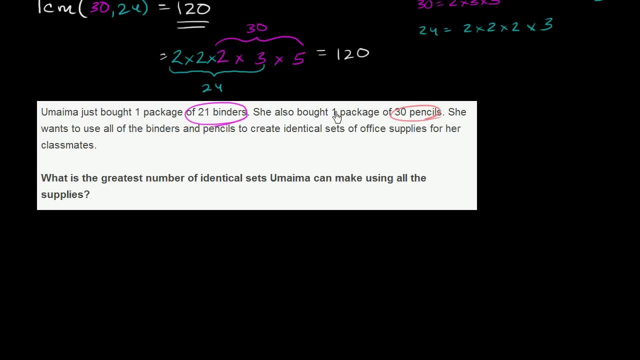 We want to divide these both into the greatest number of identical sets. So there's a couple of ways we could think about it. Let's think about what the greatest common divisor of both these numbers are, Or I could even say the greatest common factor. 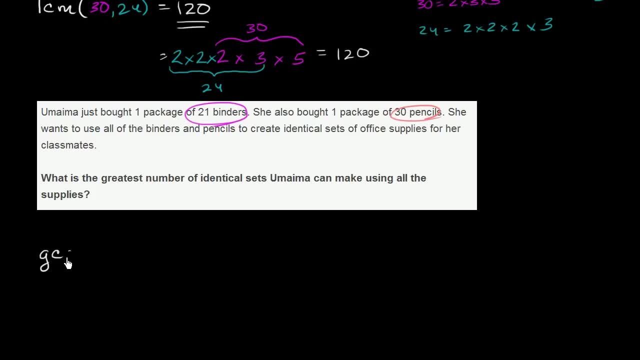 The greatest common divisor of 21 binders: 21 binders, 21 binders 21 and 30. So what's the largest number that divides into both of them? So we could list all of their normal factors and see what is the greatest common one. 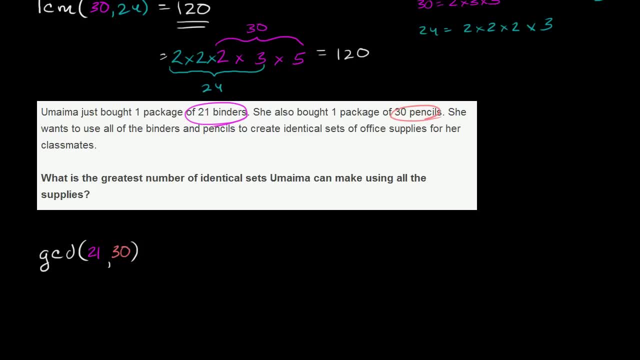 Or we could look at the prime factorization. So let's just do the prime factorization method. So 21 is the same thing as 3 times 7.. These are both prime numbers. 30 is 3.. Let me check it right. 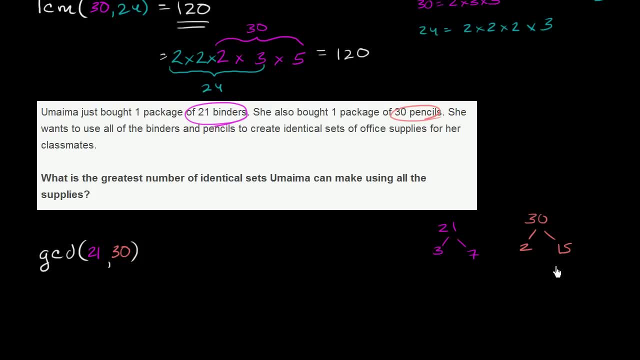 This way, It is 2 times 15.. We already did it, actually just now. And 15 is 3 times 5.. So what's the largest number of prime numbers that are common to both factorizations? Well, you only have a 3 right over here. 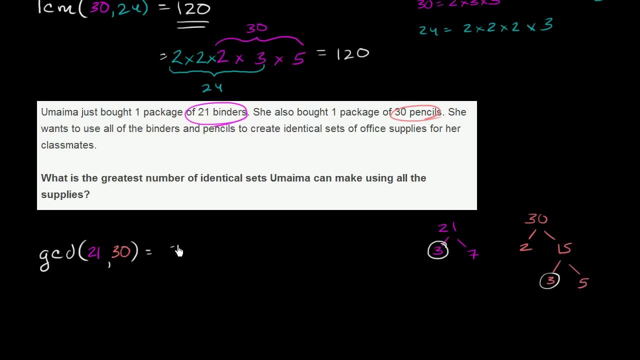 You don't have a 3 times anything else, So this is just going to be equal to 3.. So this is essentially telling us: look, let's divide both of them. We can divide both of these numbers into 3. And that will give us the largest number of identical sets. 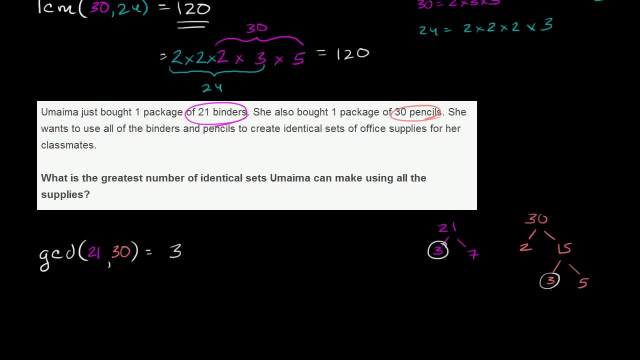 So just to be clear what we're doing. So we've answered the question. It's 3.. But just to visualize it, for this question let's actually draw 21 binders. So let's say the 21 binders So 1, 2, 3, 4,, 5, 6, 7, 8, 9, 10,, 11,, 12,, 13,, 14,, 15,, 16,, 17,. 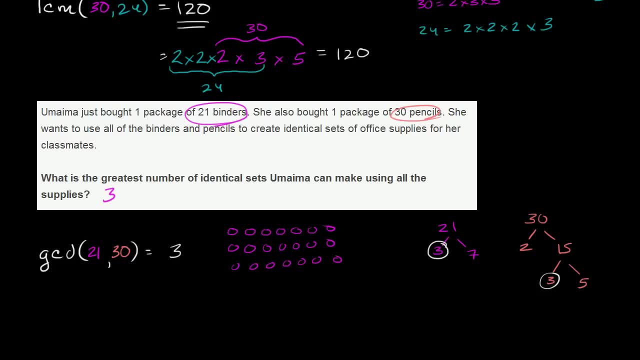 18,, 19,, 20,, 21.. And then 30 pencils, So I'll just do those in green. So 1, 2,, 3,, 4,, 5,, 6,, 7,, 8,, 9,, 10.. 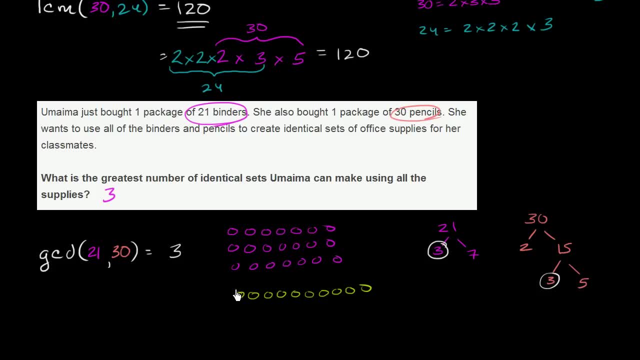 And then 20.. Let me just copy and paste that because it's getting tedious. So copy and paste. So that's 20.. And then paste: That is 30. Now we figured out that 3 is the largest number, that